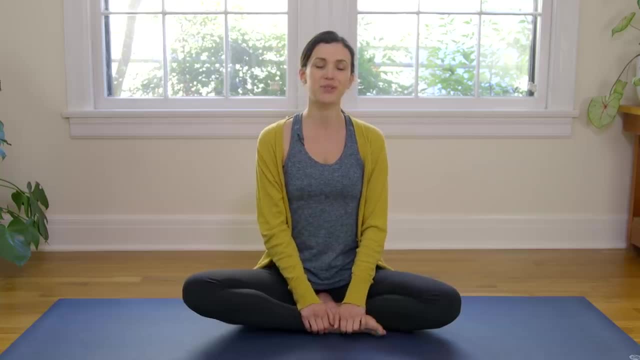 for focusing on sensation over shape, which is important. If you're a regular member of the Yoga With Adriene community then chances are you've heard me say it before: a little goes a long way. And if you've practiced even just a little bit, 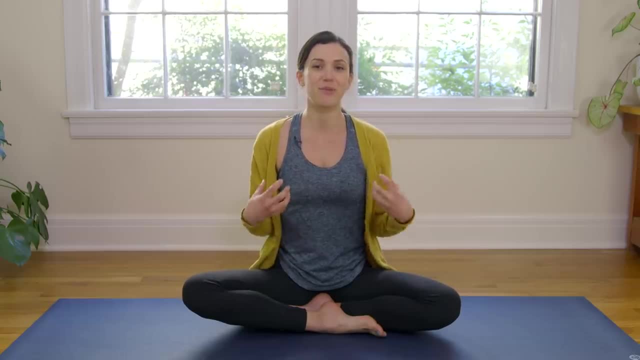 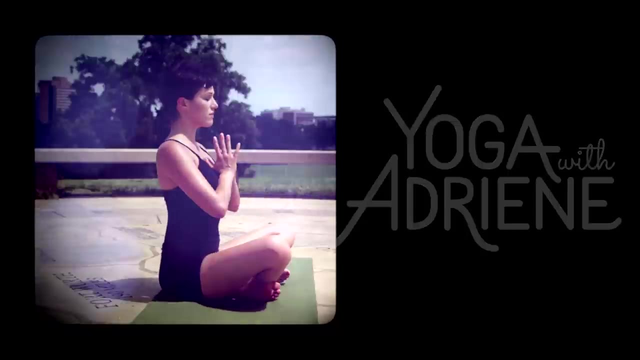 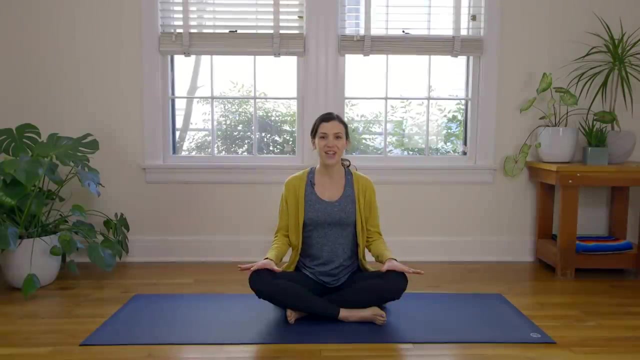 I'm sure you'll agree. So let's hop on the mat, check in with where we're at today. Let's get started. Alrighty, let's begin in a nice comfortable seat. Depending on where you're at today, you could even start this part on your couch or in a chair. 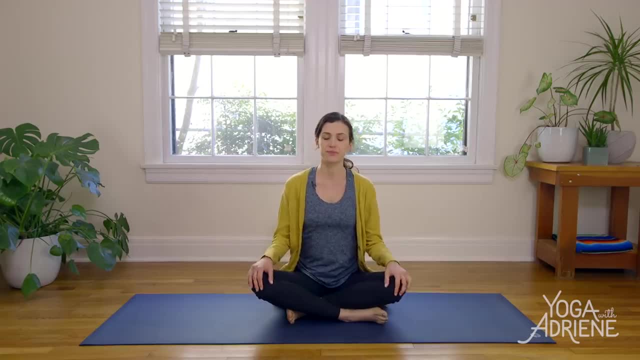 So truly find a place where you can get comfortable, Because we're gonna start with some pranayama, some breath work, breath practice, And this can be a little tricky, especially if you're new to the practice, Because I think a lot of times people don't consider. 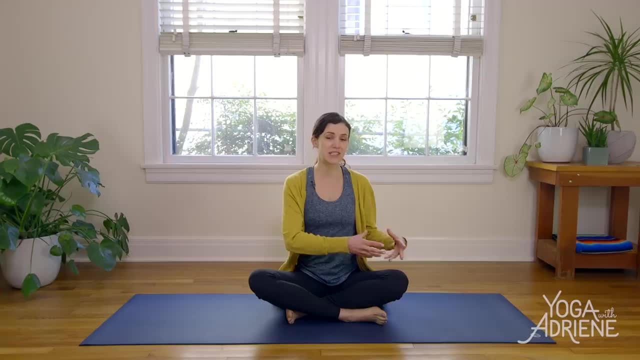 or know, have an experience that the breath practice is as challenging sometimes as the asana practice. They are part of one. It's a physical practice, the physical branch of yoga. So if it's hard for you to settle in, I guess I'm just saying you're not alone. 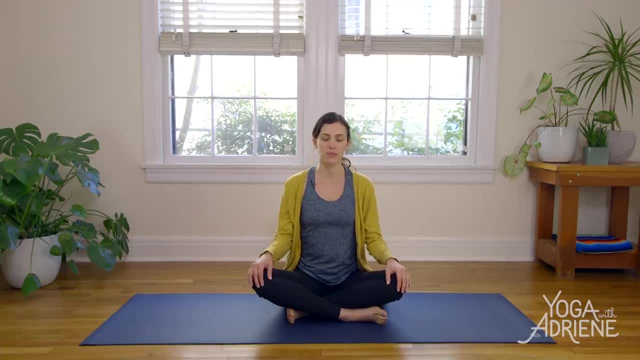 Let's give it a try, because with the breath we can really change our game. So the theme of today is a little goes a long way And just taking, you know, I mean we know this right, Intrinsically, intuitively, taking one deep breath. 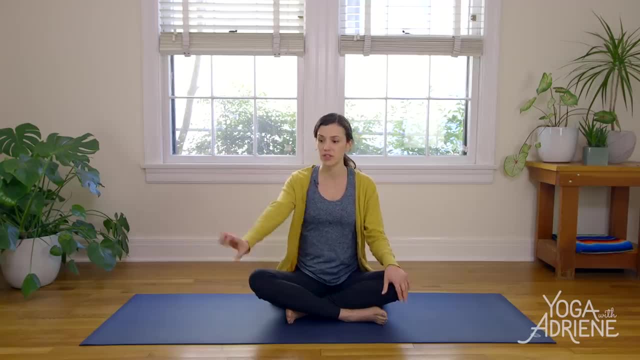 at a certain point in your day- whether it's in traffic or when you're dealing with someone or you know can happen. It can absolutely support you in that moment. It can totally be a game changer. So, that said, come into your comfy seat. 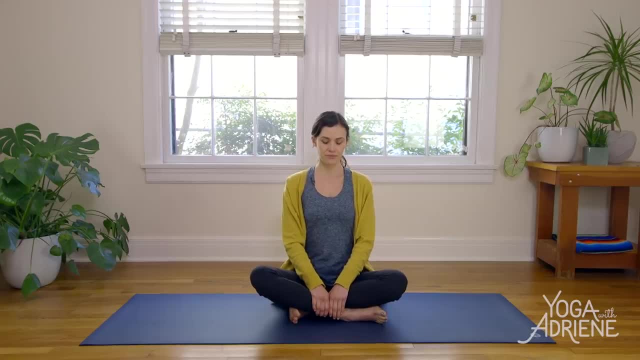 And sit up nice and tall And then just allow your energy to kind of land here And maybe put the hands wherever feels good. So be really mindful about where you are placing the hands, just as a way of spreading a little awareness out. 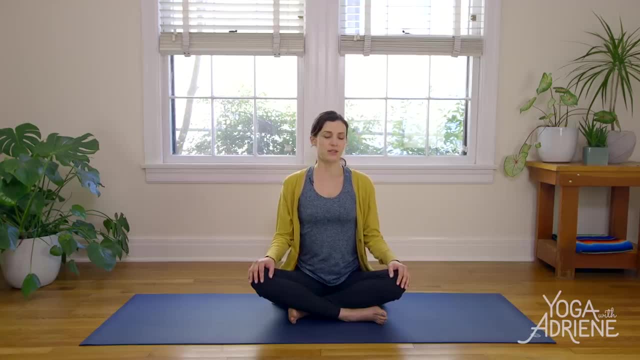 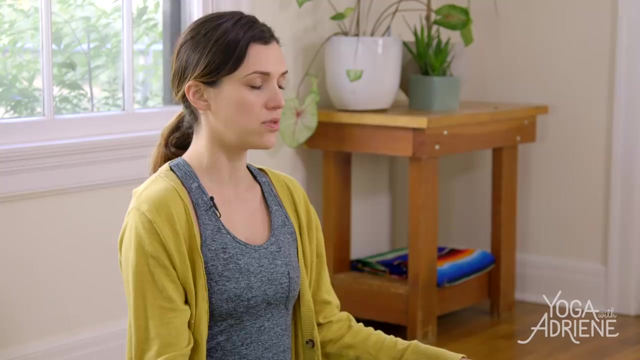 Spread awareness out to all parts of the body, Sit up nice and tall And we're not gonna do anything, in particular today. So nothing fancy, Just a couple moments of deep breathing, alright. So no fancy pranayama, Just really conscious, full, deep breaths. 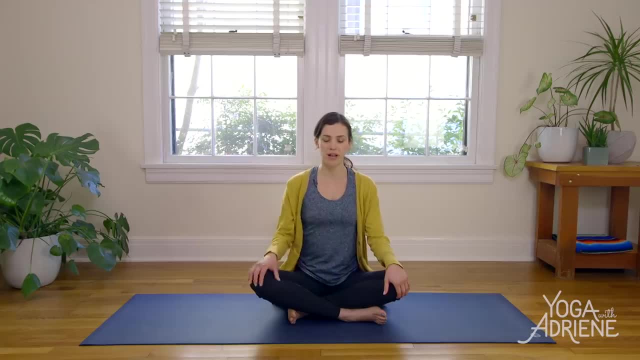 So we'll do about 10 of them, But don't worry about the number count. Just close your eyes. I'll breathe with you. Keep lifting up through the crown of the head, Sit up nice and tall And then, after about 10 or so breaths, I'll cue us. 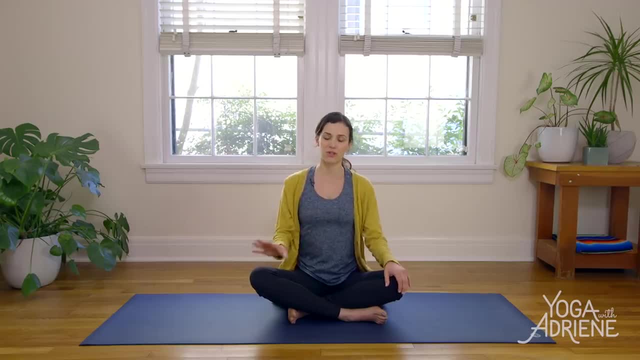 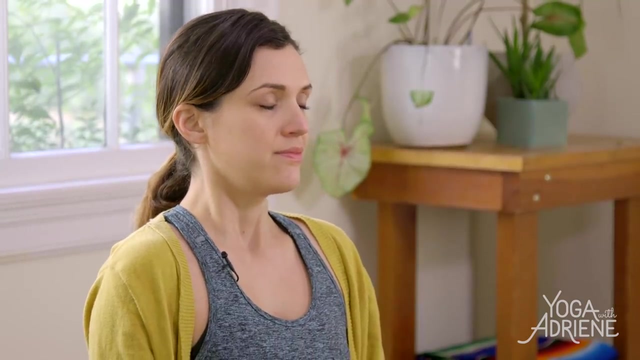 So you can kind of trust the video, trust me, trust yourself and close your eyes. Here we go, Sit up nice and tall And we'll begin to deepen the breath, So big, conscious breath, in Mindful release, Just as you exhale out. 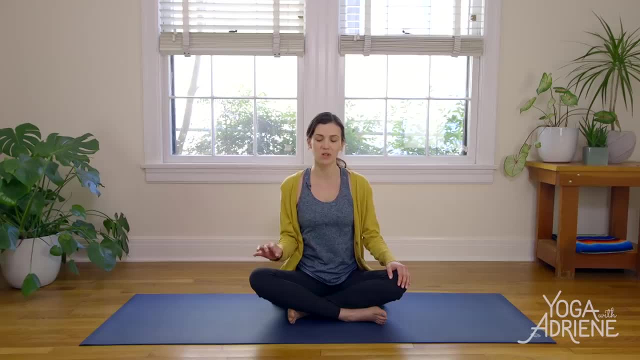 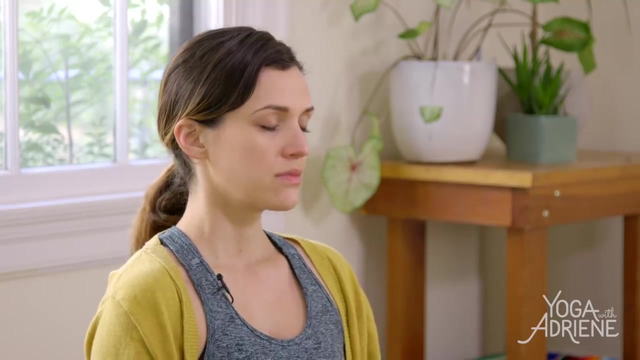 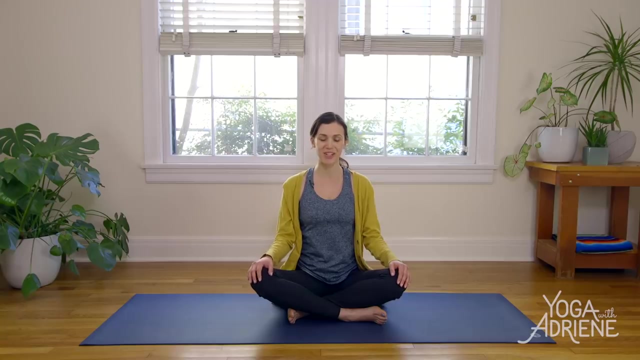 And see if you can slow your breath down a bit, Make the inhalations a little bit longer and smoother, And same for the exhalations, Just as you exhale out, And then notice where your thoughts have gone, where the mind goes. 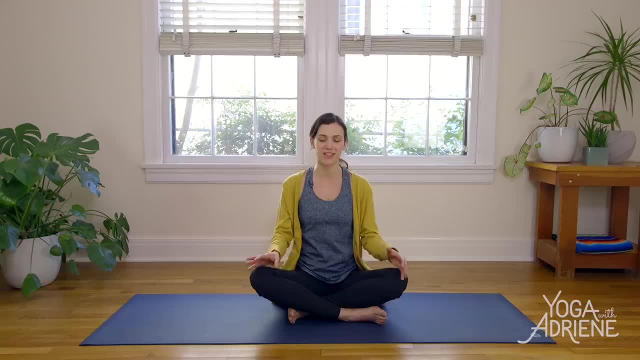 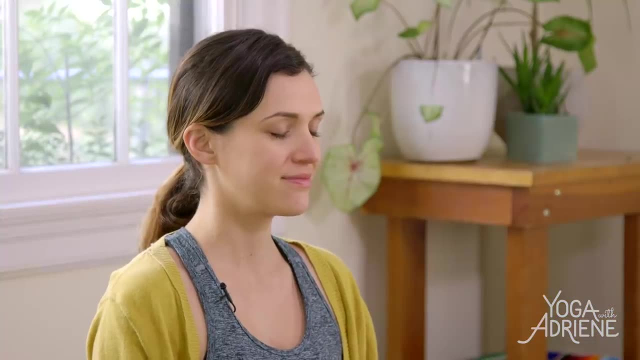 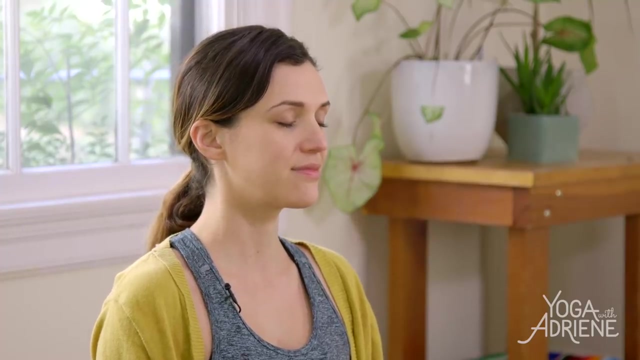 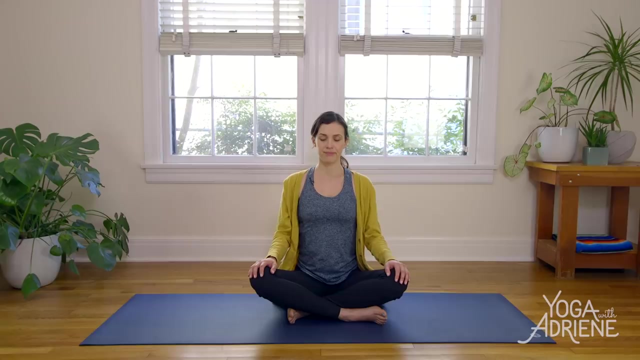 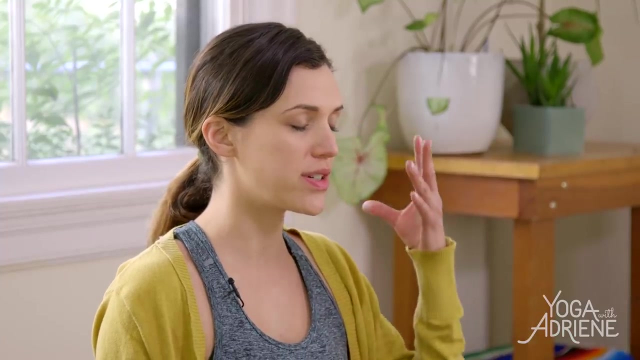 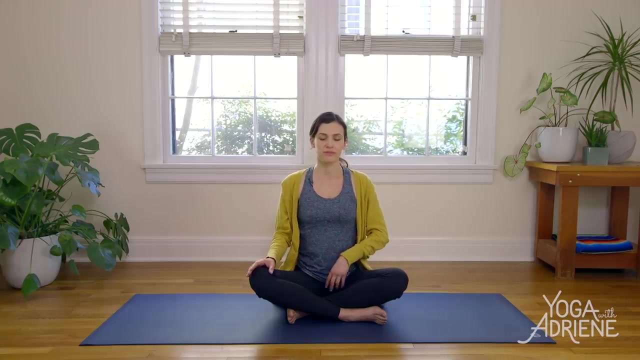 And just notice that, acknowledge that, and then come on back to the breath practice. We're breathing deep here, Deep breathing, And on your next inhale imagine the breath coming in through the nose and traveling down. So the direction of the breath is down as you inhale and then it does this kind of 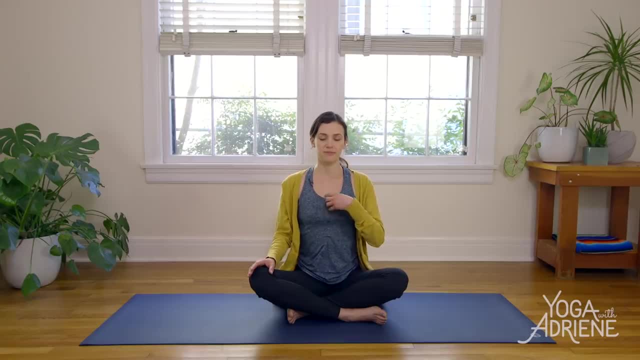 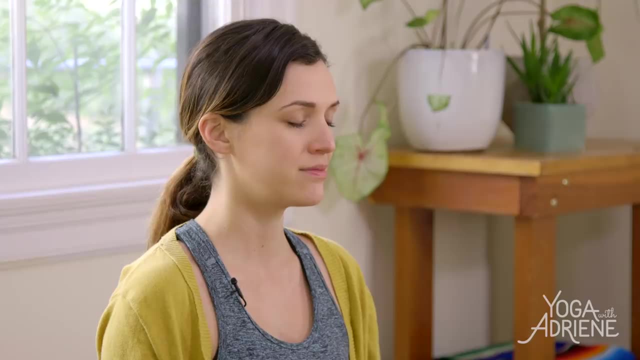 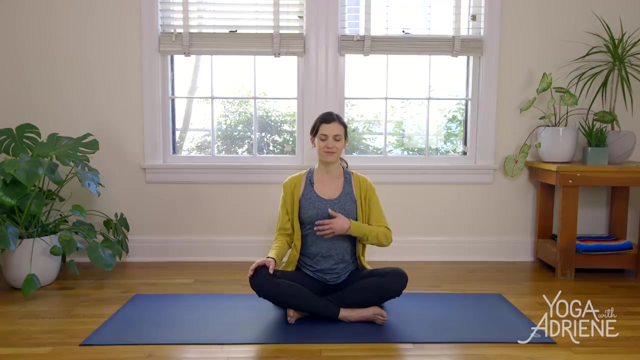 sweet little somersault and then comes up as you exhale. Let's try that one more time: inhale, breathing down, and then exhale. breath travels up and out through the nose, Great Bat the eyelashes open, loop the shoulders and we'll let that go. 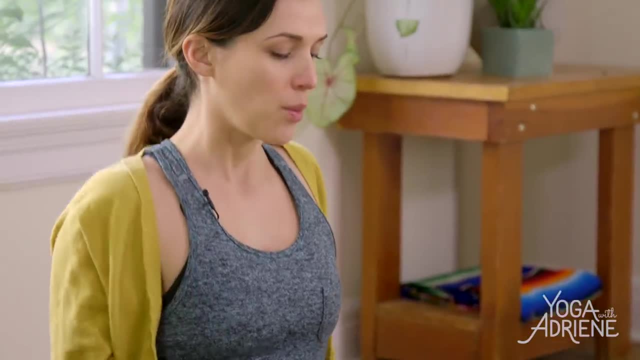 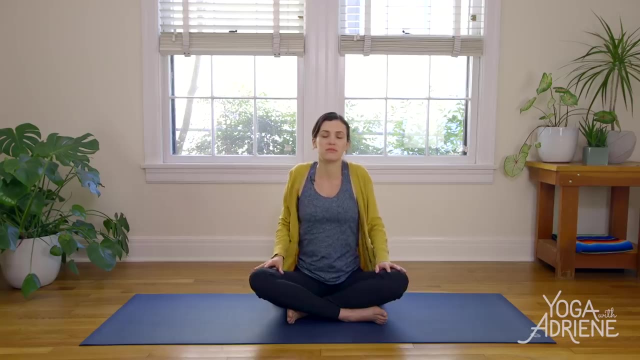 So it doesn't mean we're going to stop the conscious breathing, But we're going to kind of let the movement in the breath become one. when two become one, Is that Spice Girls? So big looping of the shoulders. If you are on your couch or in a chair, now go ahead and come onto the ground. 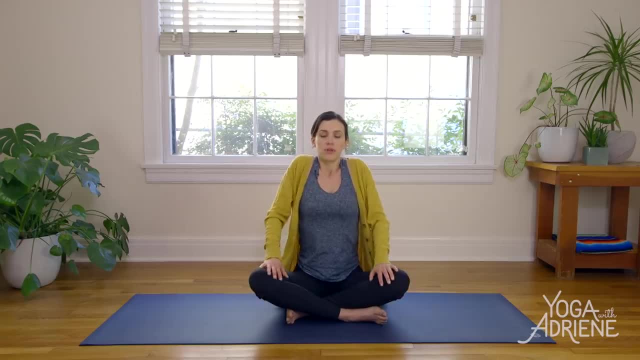 Maybe have a yoga mat, maybe just onto the floor. We'll come into a nice comfortable seat. So keep conscious breath going, whatever that means to you. Keep coming back to a nice deep inhale, nice long exhale, whenever you can. 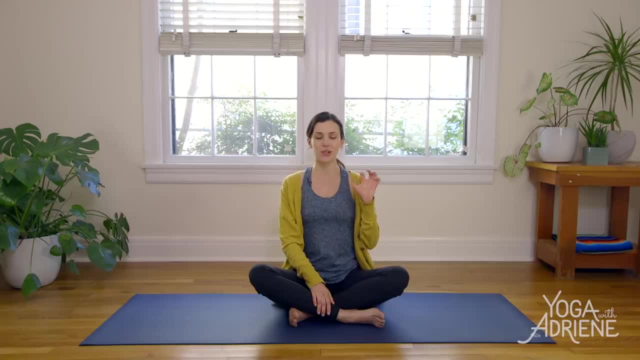 Little goes a long way there. Sit up nice and tall. We'll take the left hand. just spread it super wide, rotate the left wrist and then go ahead and place it on the ground and inhale. reach the right fingertips up and overhead. 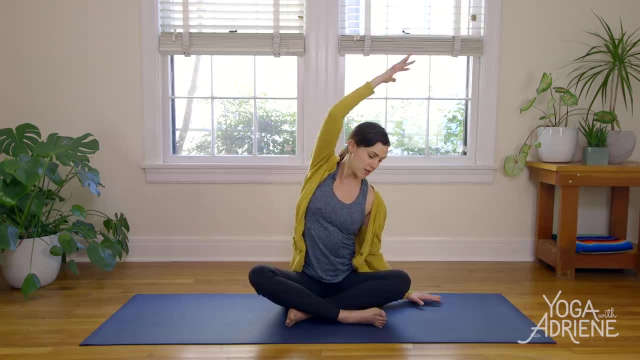 Side body stretch. so good, A little goes a long way here. so find a little movement, whether it's gentle, pulsing, maybe it's opening the chest Towards the sky and then rounding it down to the ground, checking in with the shoulder. 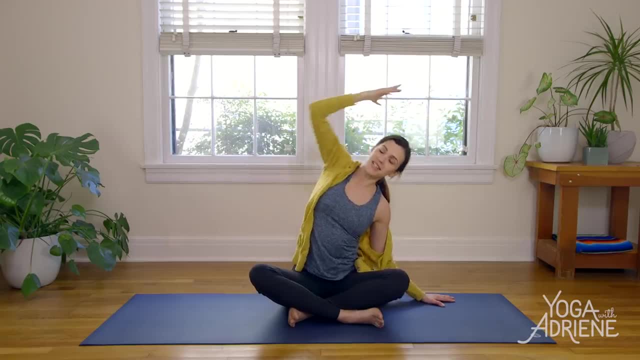 Find your deep breath here and then come back to center. I do declare and then, right hand, spread the palm super wide, rotate the wrist. This is great if you sit at a desk, just kind of opening up, through the hands, the wrist. 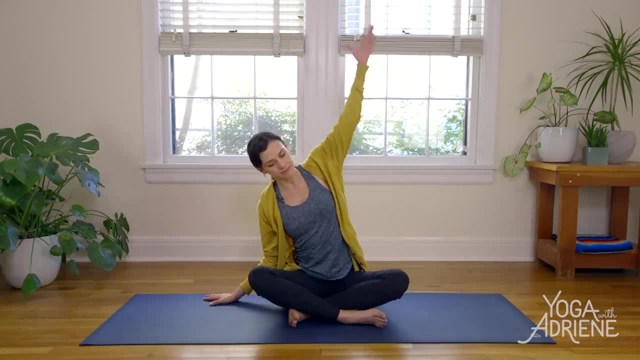 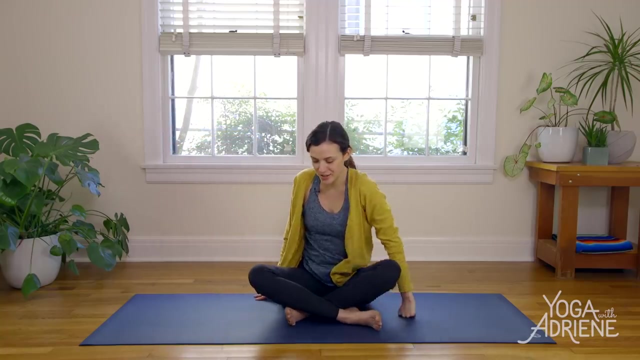 and then side body uncrumbling- Great for lower back pain too. Remember it's all connected. Find movement that feels good here. See if you can keep up with a conscious breath, Great. then come back to center and send your legs out long. 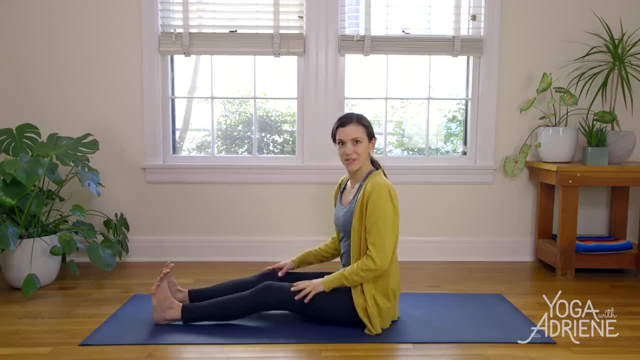 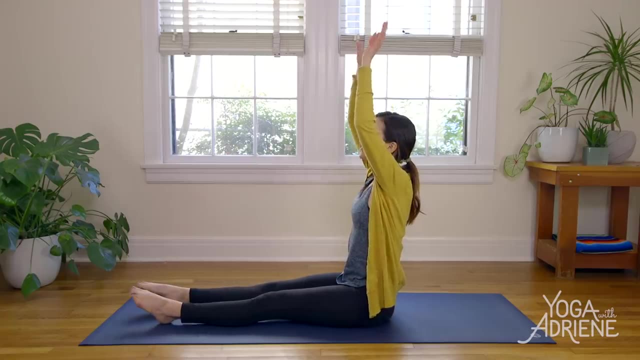 I'm a little sore Firming down through the tops of the thighs. nothing fancy here. Reach the fingertips up As you breathe in and then forward fold as you breathe out. Even if you only land here, you're great Way to be where you're at today. 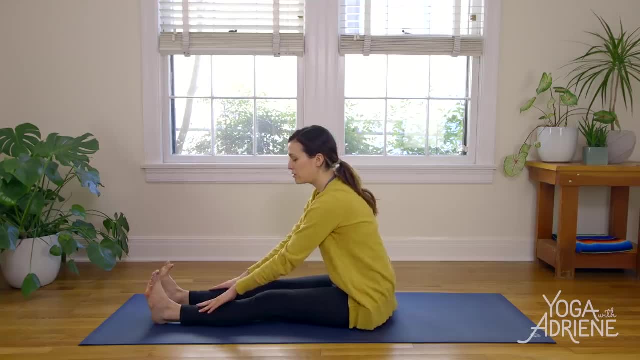 You need to breathe into the back body, stretch, stretch, stretch. Don't feel like you need to push it to any certain shape here. Focus on the sensation over the shape. Find your version of this here and then connect to your breath. 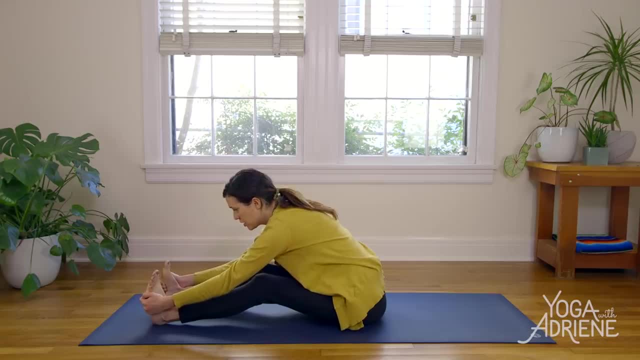 This is also good standing. If this is too tricky, It's okay, It's okay, It's okay. You can do a standing forward fold instead of a seated forward fold, And that one you can do anytime anywhere. Just be careful when you do it in the shower so you don't slip. 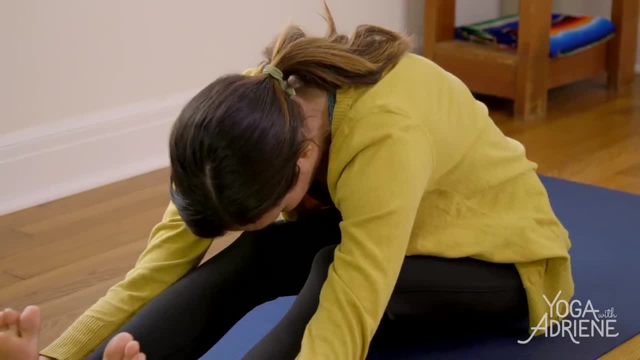 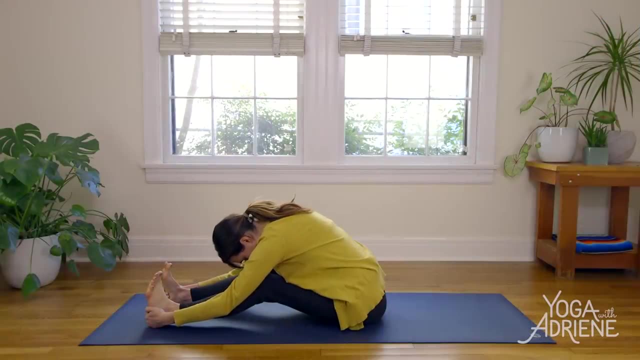 Wherever you are, whether you're seated or standing here, forward fold, Allow the weight of the head to relax and release down. This is an awesome pose to check in with daily, Not just for the muscles of the body, But for the nervous system, for the mental aspect to your practice. 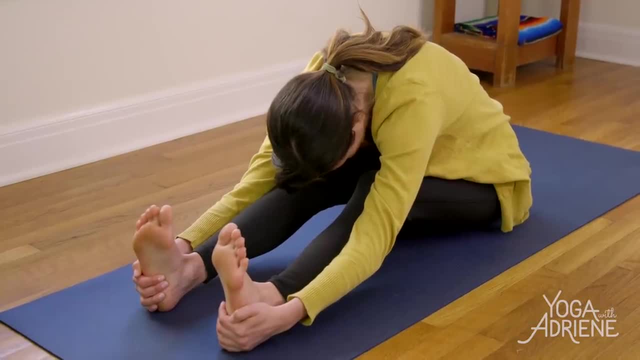 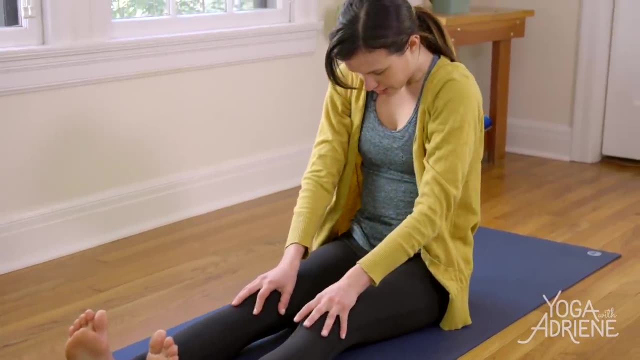 Then connect to your sitting bones If you're seated, if you're standing, connect to the soles of your feet, All four corners And everyone. tuck the chin into the chest and roll it up. Great, Just in case you took me up on the standing, come on back down to seated. 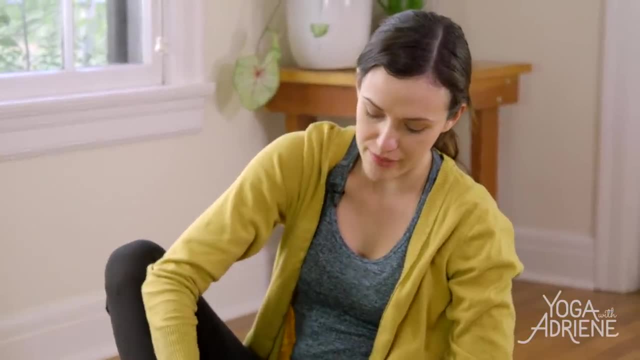 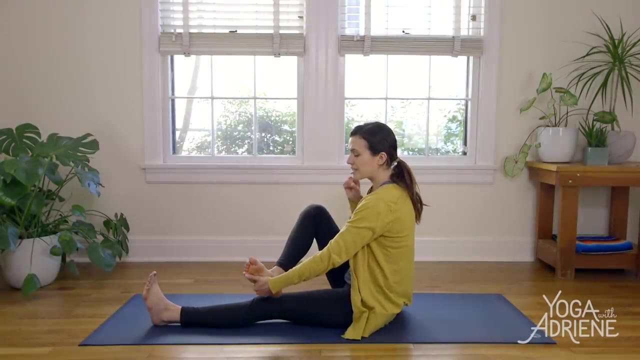 And just nice and easy. we're going to take the right foot into the left palm. So start here. Be super mindful here, especially in these little yoga breaks. You can never be too mindful, because it's always kind of in those unthoughtful moments. 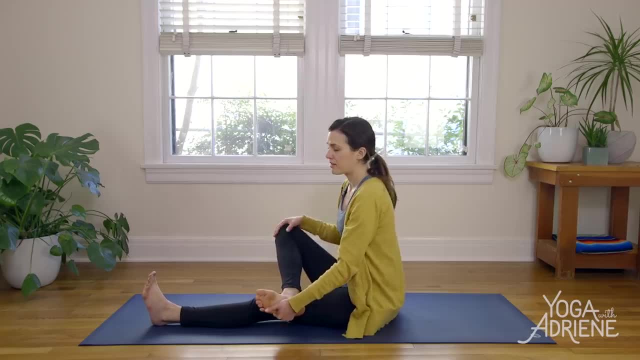 that you end up kind of tweaking something or anything. if ever So, it's usually not in the actual yoga practice, at least with my community of friends, where people get injured. It's always kind of in the moments in between. So stay present. 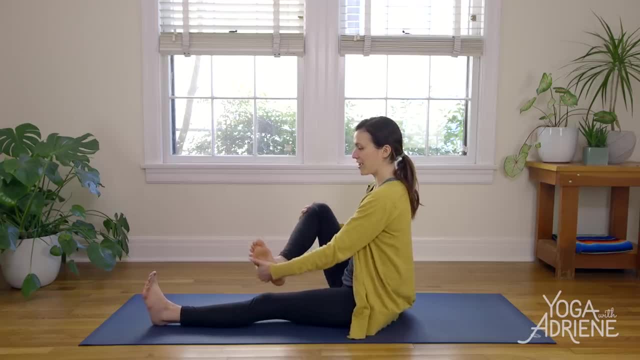 And we're going to come to a little rocking of the cradle, of the leg and the foot. Okay, Sorry, Right hand comes to the outer edge of the right knee And this will be a little different for everyone. If you're like I can't grab my foot. 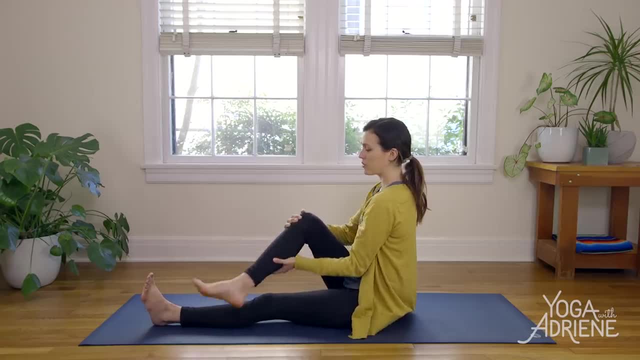 No worries, Just grab your calf here. And so what again we're focusing on is the sensation over the shape. So unfortunately, I mean I don't want to be negative, but unfortunately- we see a lot of instructors Just kind of slamming into the shape because it's in their body and then it's hard to decipher. 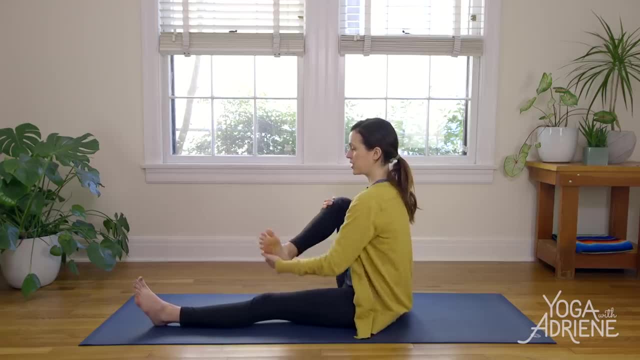 what it is for us. So it could be this for you. It may not be this, Okay. On the same token, if you need a deeper stretch, go ahead and bring that right foot into the crease of the elbow, the left arm. 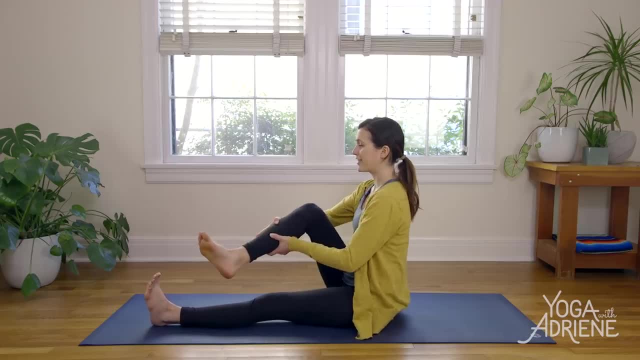 You can come here. So we're here or we're here, or we're here And we're imagining the ball and socket joint here on the right, in the right hip, And we're breathing and we're doing our best to sit up nice and tall. 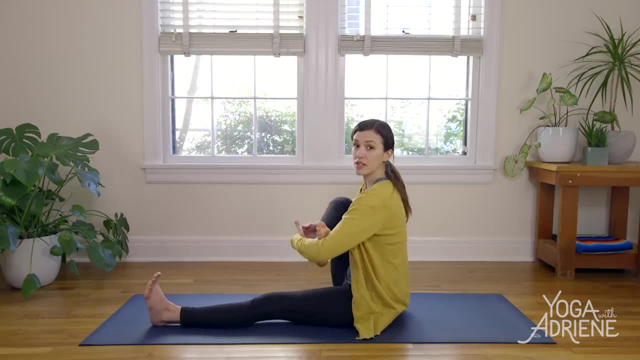 So all of these things are great, things we can do as a sequence, or great things that we can do on their own. For instance, this is a great thing to do. All of these things, actually so far, are really great to do while you're watching TV. 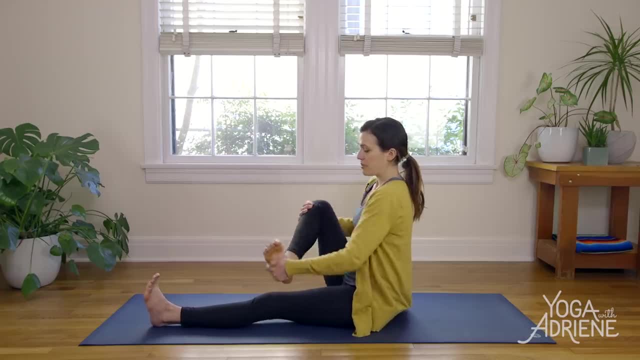 So after this video, if you're watching this on your big screen, you can pop on an episode of your favorite. See, if I had a TV show, I could send you to my TV show right now. Just kidding, Kelsey, we're working on a TV show. that'd be fun, but I want all the community to be. 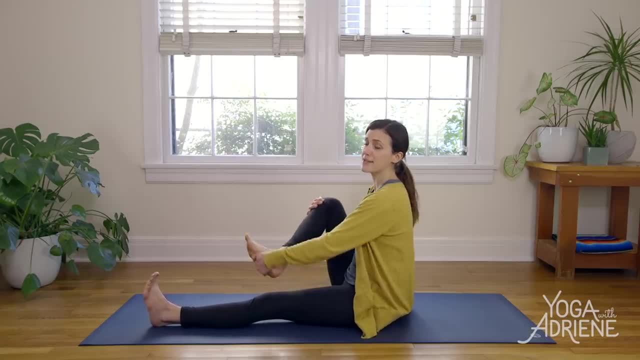 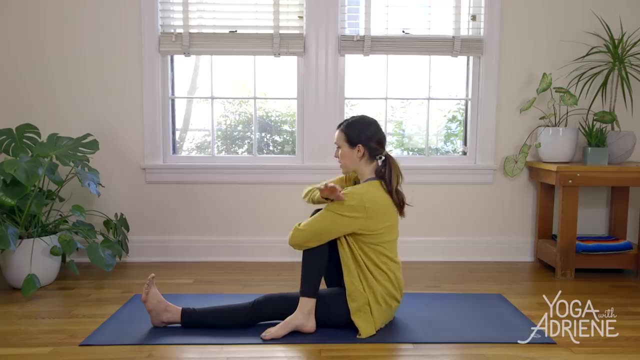 in it, Travel around and visit the community. Yes, take your right foot, cross it over. Nice twist here We're gonna hug the right knee with the left elbow, roll up through the spine, swim the right fingertips behind and boom. 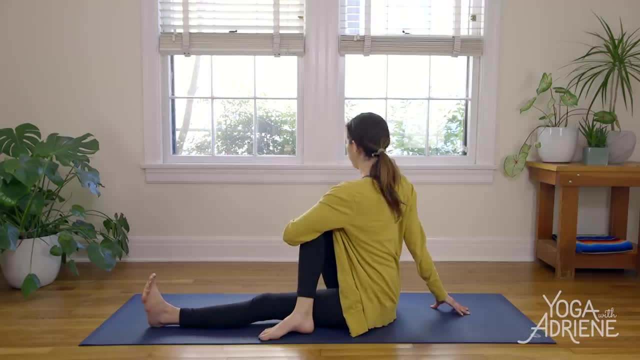 Find what feels good here, Maybe point and flex through the extended leg. So I wanted to mention It can be this twist or it could be anything. A little goes a long way with the twist Reclined twist. You always want to find that deep breath in a twist to get the full benefits. 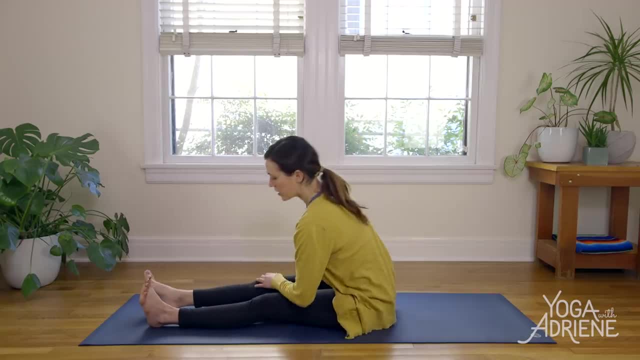 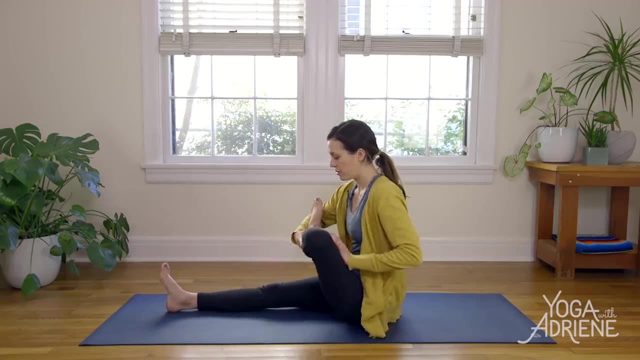 Then we'll release and switch on the other side, Switch to the other side, Bend the left knee, rock the cradle. So it's a practice. Yoga asana, we're taught shapes. That's the physical practice. So take it upon yourself with your home practice, and I think that's what's cool about Yoga. 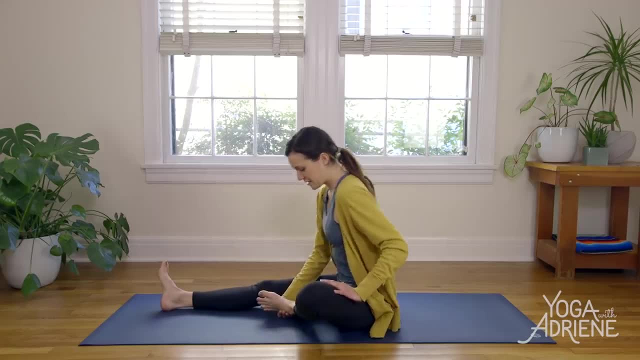 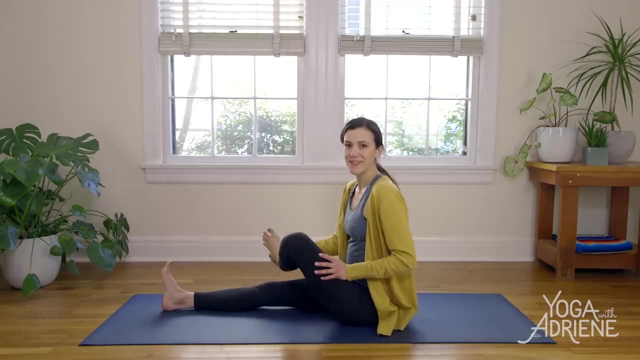 with Adriene too, because this will just help you when you go to your public class to focus on sensation over shape, and then you'll want to come back to your mat. You're gonna want to take these little yoga breaks every day. Okay, Okay. 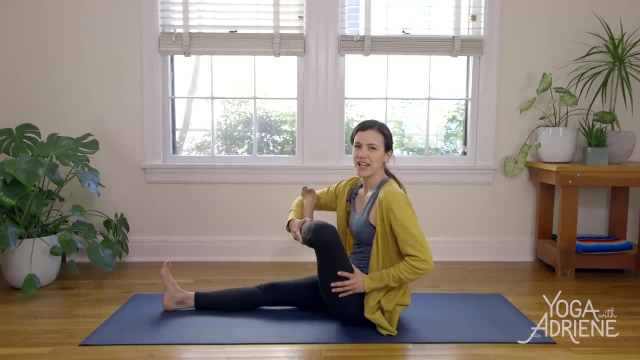 Okay, Okay, Okay. And then you stop comparing yourself to other people too. at least I have, or I try, because I'm like: no, you know, when you really focus on what feels good for you, kind of really doesn't matter what other people are doing. 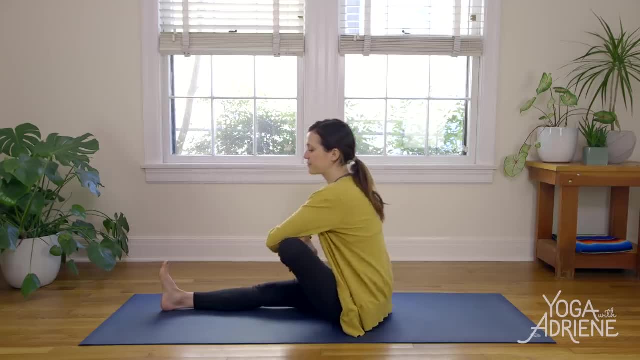 I mean, you can be inspired by someone, but This video turned into a yoga lecture by Adriene. Okay, So after you've moved around a little bit here, go ahead and cross it over into your twist. Notice if you're kind of leaning back here. 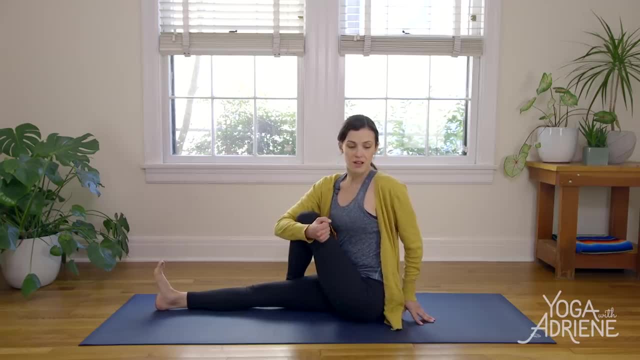 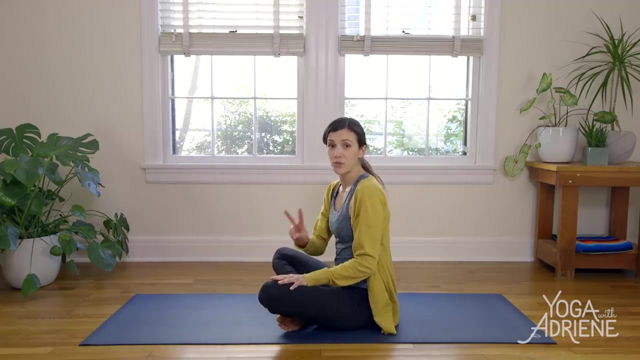 notice: if you've lost connection between your feet, Reconnect Great, And then we release, Cross the ankles, come to all fours. We have two more things to do, So you know your cat-cow, so I'm not gonna do that one. 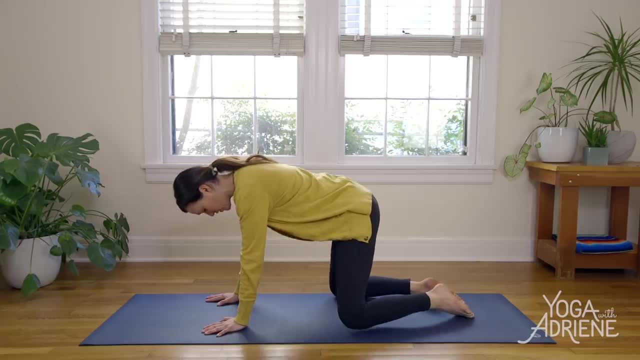 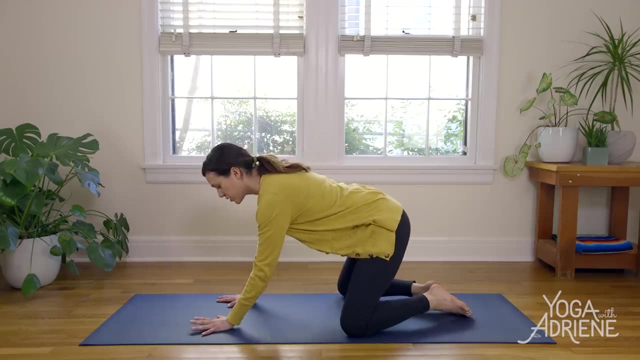 because I feel like everyone really knows that anyway And you can insert that here as a freestyle- We're gonna bring the knees super wide, big toes to touch. If you come to my public classes, I rarely do not do this. next little ditty. 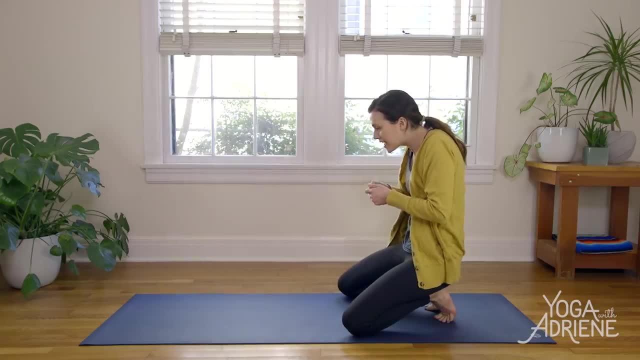 because I feel like we're constantly here with the head neck forward here here all the time. So this is, this is great little neck and upper back body hygiene. Here we go, Inhale, Reach the right fingertips forward. 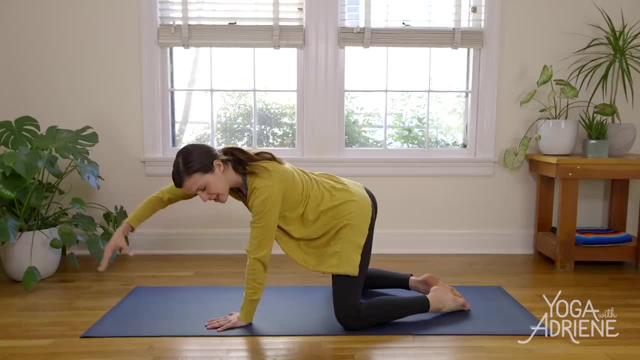 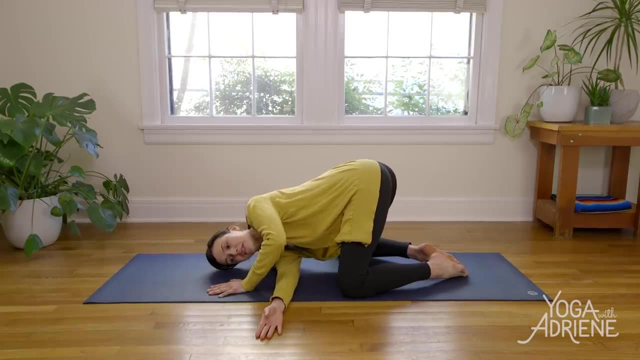 Find that length, that stretch in the right side body and then try to maintain that as you thread the needle. So right fingertips in and underneath the bridge of the left arm and we come to rest on the right ear. outer edge of the right shoulder. 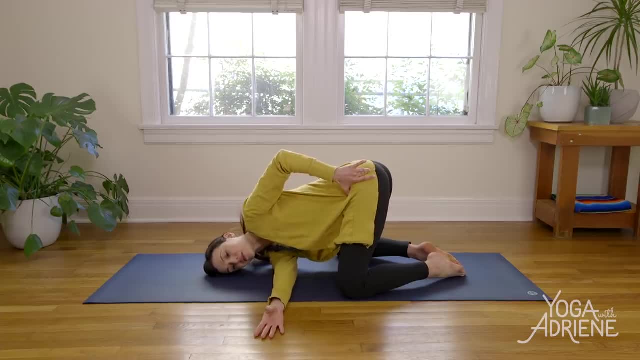 Keep a connection with your big toes and the knees are wide so that we can find this awesome rock in the pelvis here. Then breathe into the upper back body and stay connected. Stay connected through your hands So you can really use this left hand to press away. 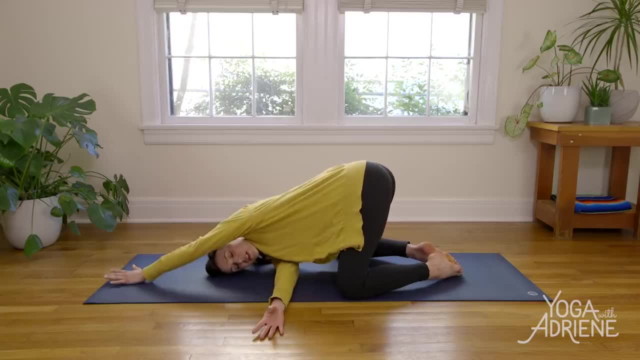 from the earth here, either by bending the elbow or finding extension. You might also like to bring it all the way up, or even around hand on the sacrum, or to twist. You know what to do here. listen to your body. 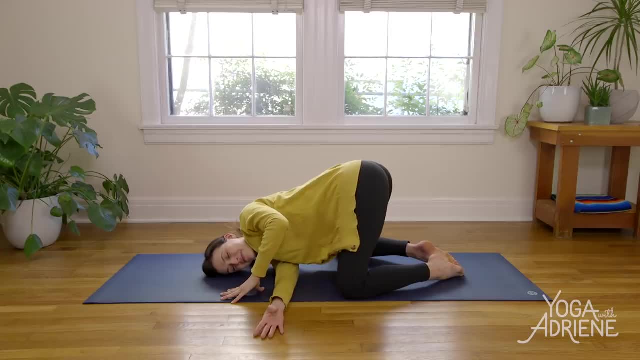 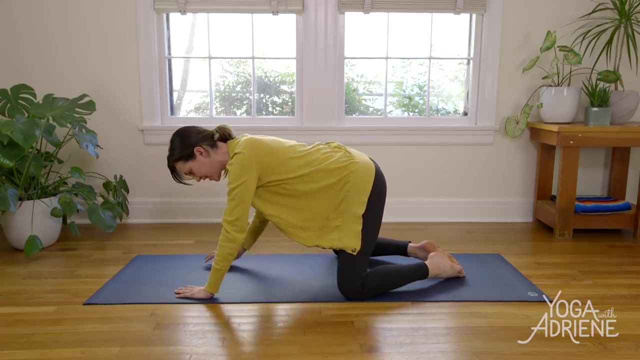 Big, deep, conscious breaths And then play with that directional breath: Inhale it travels down into the belly and exhale up and out, Then slowly release, pressing your foundation to come back again. Pay attention to the mindful moments in between. 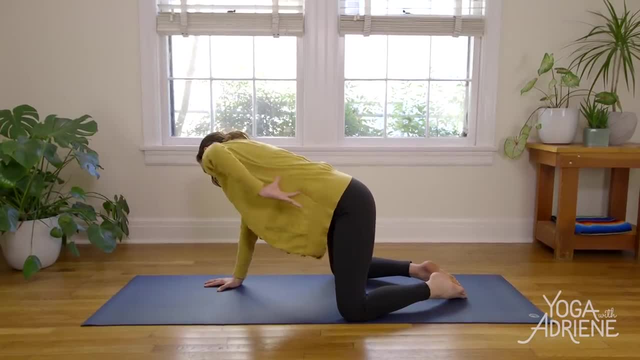 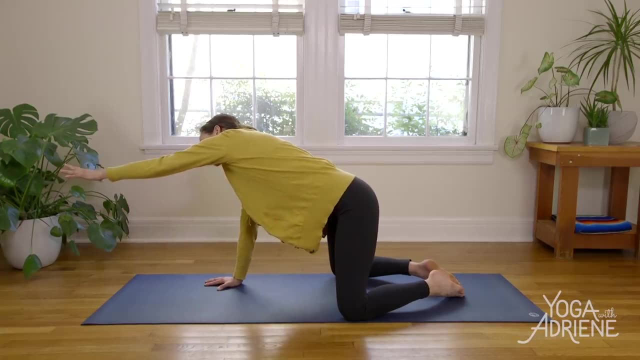 And the same thing on the other side. Left fingertips stretch, try to maintain. So sometimes when we just come into it from here, we have all this collapse in the side body. So this little bit of consciousness in the side body goes a long way as we thread the needle. 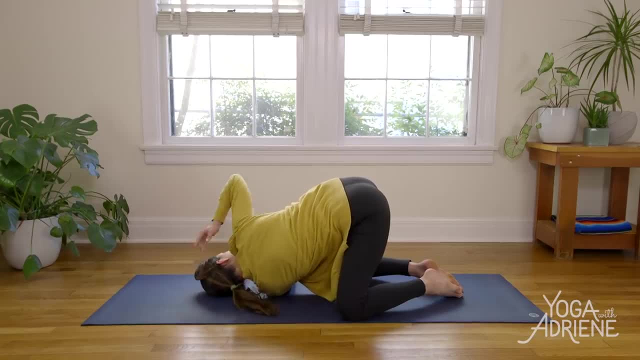 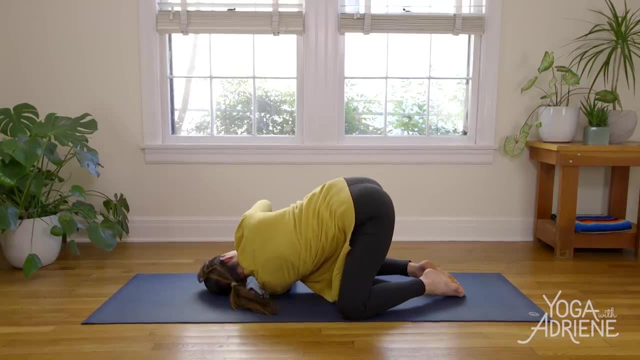 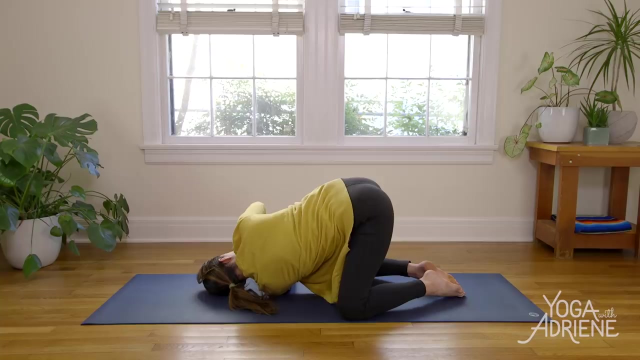 Or, excuse me, left fingertips underneath the bridge of the right arm. And same thing: try to stay connected to your toes, Find what feels good with the right arm and breathe. If it's too much, don't worry about it, but otherwise maybe you play with that directional breath. 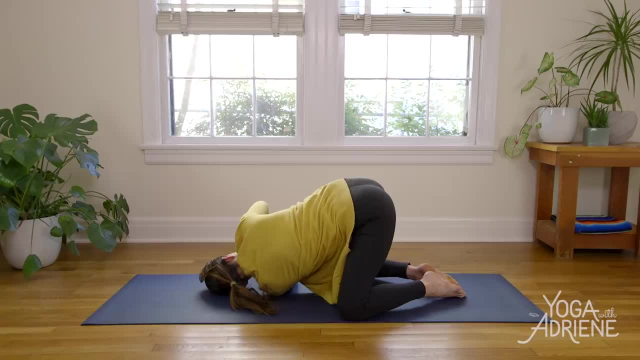 Inhaling, filling the belly with air And then exhaling, imagining the breath traveling up and out the nose or the mouth. Sweet, one more breath And beautiful release. I always love my view from here Depends where I'm at and which day. 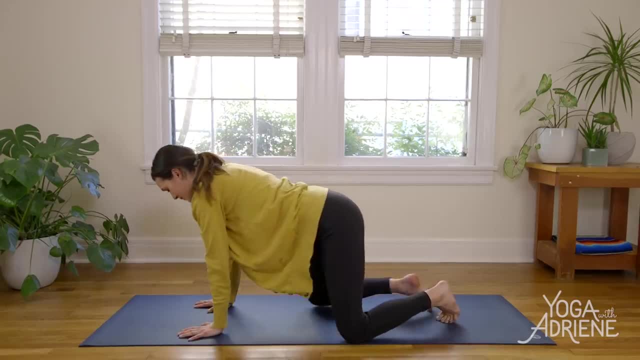 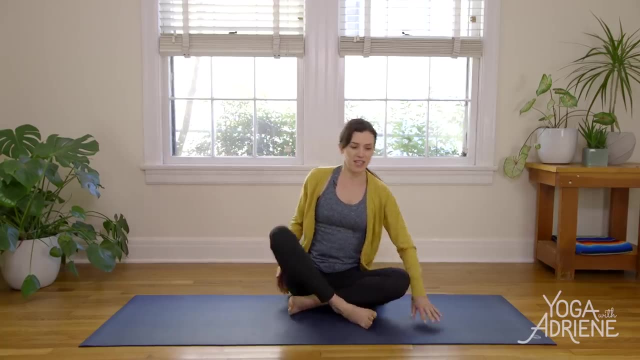 but today is really pretty Okay. coming back to seated, You can also do this one standing. If you've done a Yoga With Adriene video, you've probably done this one standing. I recommend doing this one standing. You've probably done this before. 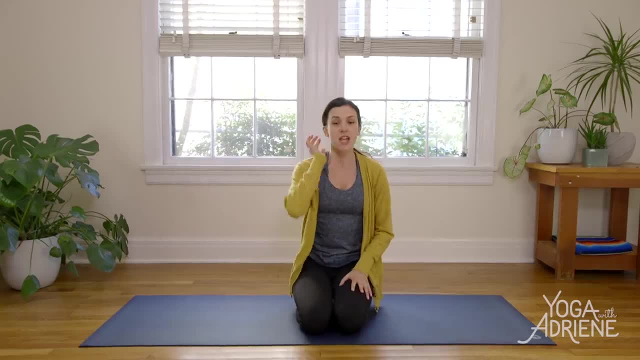 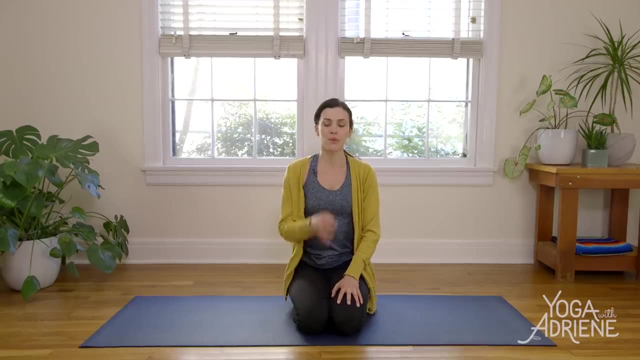 I'm actually gonna come to my knees. Neck circles, Not 1980s neck circles, as fun as they were, are Okay. we're putting this is what we say in kids yoga, but it works. we're putting a little marker here. 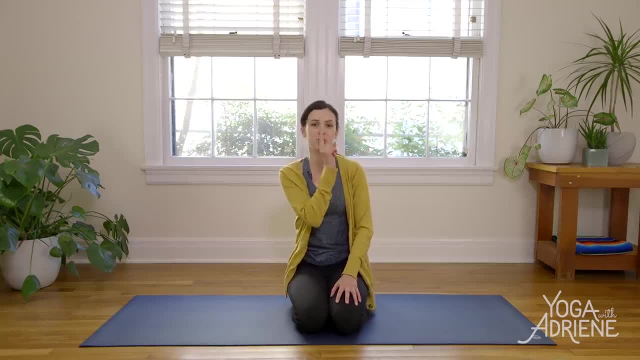 You can choose your color Or, if you're sophisticated and modern, you can put a little charcoal pencil on the tip of the nose And we're starting with small circles today. So small, tiny, tiny circles: Head over heart, heart over pelvis. 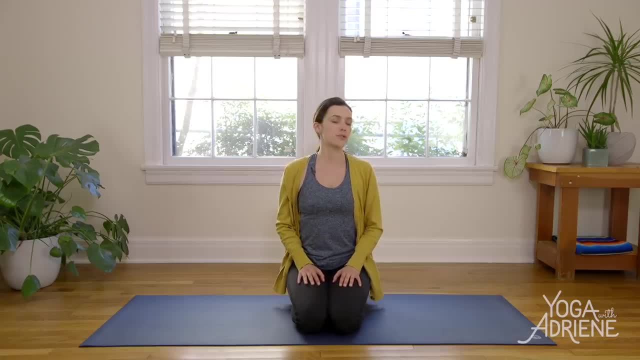 So sit up tall or stand tall And then allow your circles to grow larger And you really need to kind of drop what you look like here and really focus on the sensation here to find that yummy spot. I'm a great example of that. 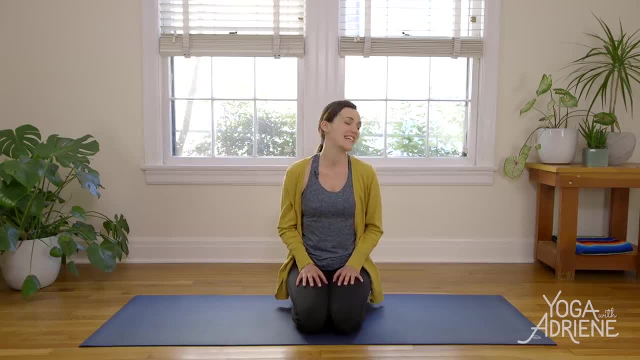 Sometimes I'm just like in public, like oh, And then allow the circles to grow larger. So we start at like button size and then we move to like full dinner plate size And you can move through like saucer salad plate, dinner plate. 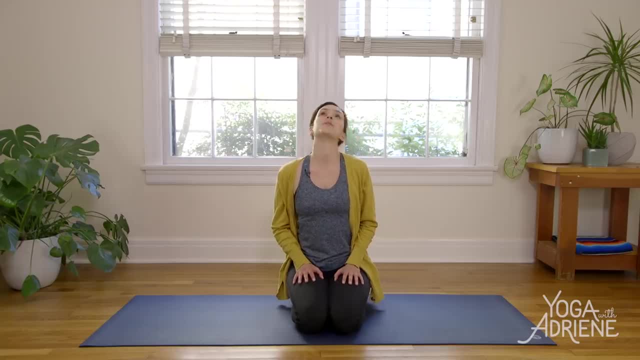 And then reverse your circle, Check in with your breath, And then, if you find a catch, you might rock a little bit in that place. You might notice that the shoulders have started to creep up out of just our habitual self, And so relax your shoulders. 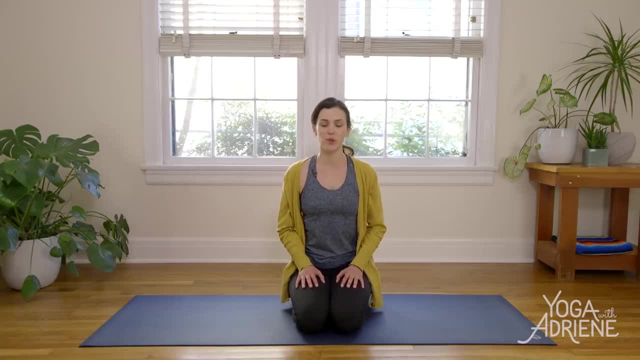 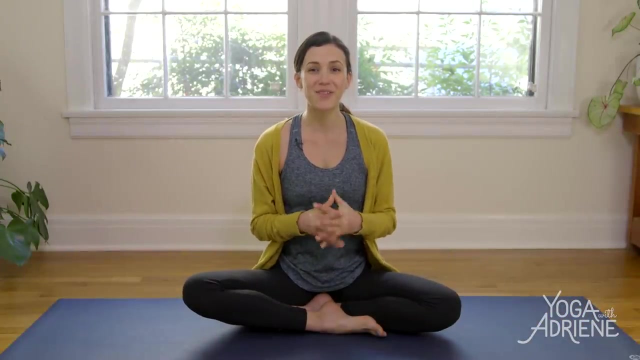 And then bring it back to center, Throw all the palms together, Big breath in, Big breath out, And then you're good to go. Okie doke, my friends. So that was A Little Goes a Long Way. I encourage you a little friendly invitation. 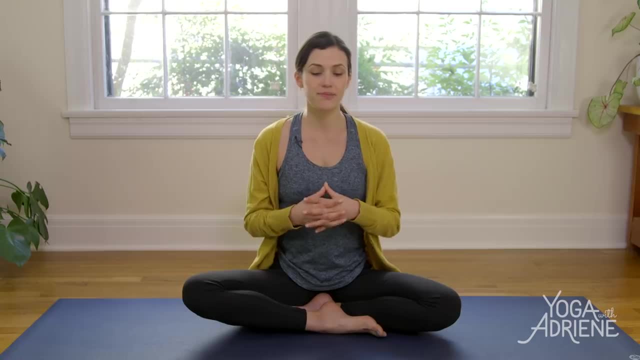 to try this once a day for a week, And I think the big idea here is that you make sure to take time for yourself and that you don't always need a big, fancy, sweaty yoga practice to do that. Sometimes, just a little bit goes a long way. 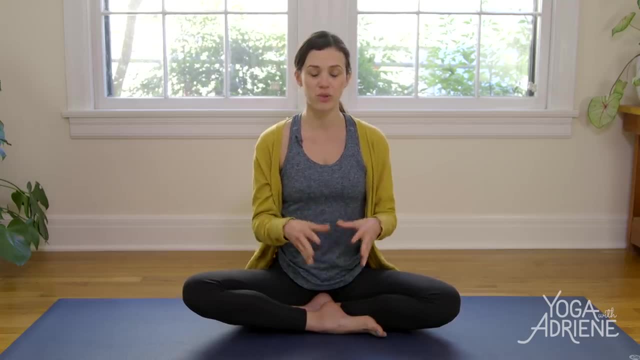 So if it's just doing one pose or one little ditty from this practice, or returning to this video every day for, say, seven days, I encourage you schedule it in your planner, whatever you need to do, Just like you would schedule anything. 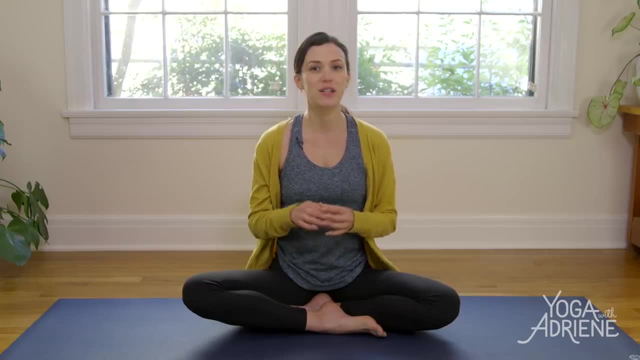 You wouldn't skip eating, You wouldn't skip a shower. See if you can touch on a little bit of this every day for a week and let me know how it goes. okay, I know it's a challenge, so handing you a friendly challenge. 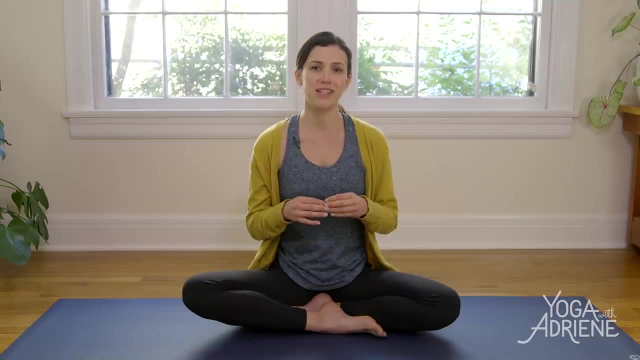 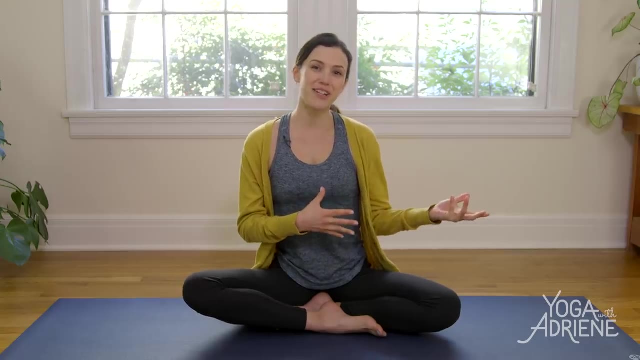 See if you can schedule time for seven days to drop the pin and find what feels good. alright, I love you guys. Leave questions, comments below. Share this practice with your friends. This would be a good one to share with someone who's new. 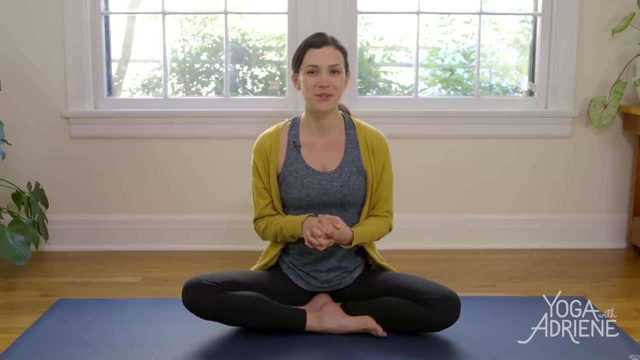 to the practice and I'll see you next time for yoga videos every Wednesday. Take good care, Namaste.